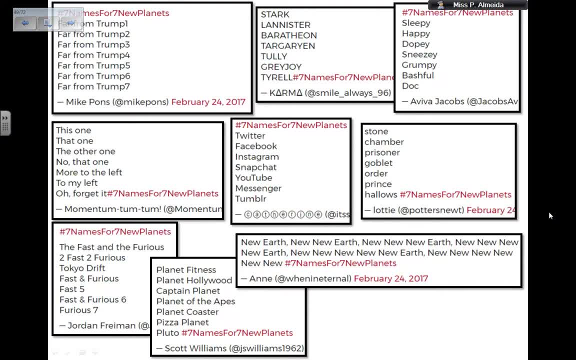 this topic, so let's get started. so, extra solar planets. i'm actually going to start with this, which is, as you may remember, um, in 2017, there were, uh, new planets, seven new planets all found, uh, in another solar system, okay, or around another star. so they are extra solar planets. the the word. 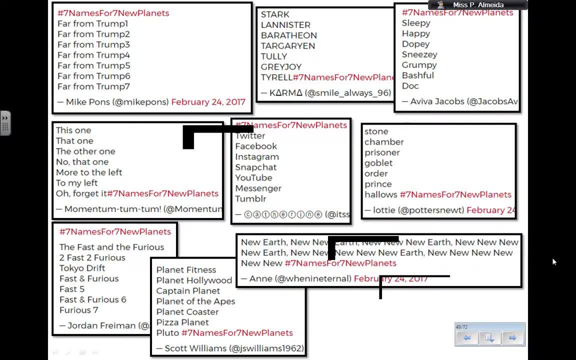 extrasolar planet or exoplanet, comes from a planet that is around another star that is not ours, so not the sun, and nasa actually asked people: uh, you know what should we name them? that we have a whole solar system there, or at least seven planets. it's quite a multiple planet system. so give us the names and 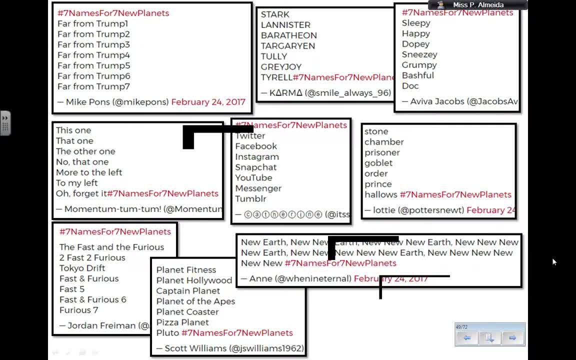 on Twitter and they were giving the seven names for the seven new planets and these are some okay. so we have the far from Trump one, two, three, four, five, six and seven. we have the start, the Lannister, the Baratheon, all of these so Game of Thrones ones. we have the Snow White's right, the Harry Potter stone. 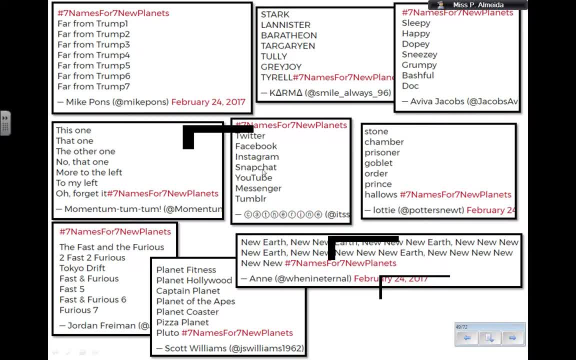 chamber prisoner, all that stuff, the social media planets, that one, I don't even know what, what to call it- the Fast and Furious range of series of movies. actually, now we would have to find more planets: the new word, new, new word, new, new, new, new word, as so, so on, and then all the other planets. so this is you. 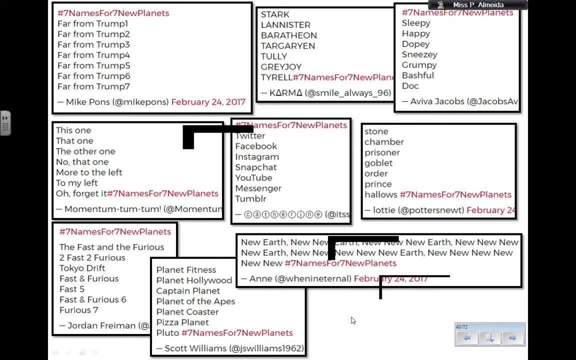 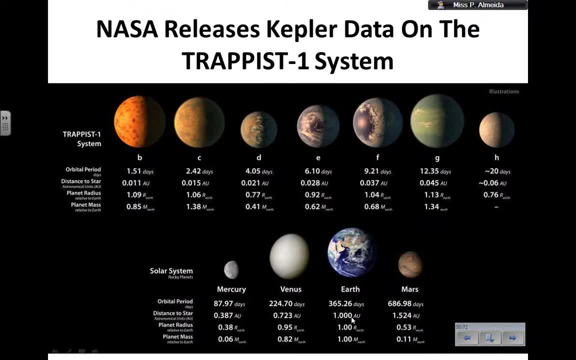 know just a little bit for you to know what one went around, but this was actually quite fun. but now actually kicking in on the video, so these were the planets, okay, and most of the planets that we are finding so far. they seem to be different than the planets that we are finding so far. they seem to be. 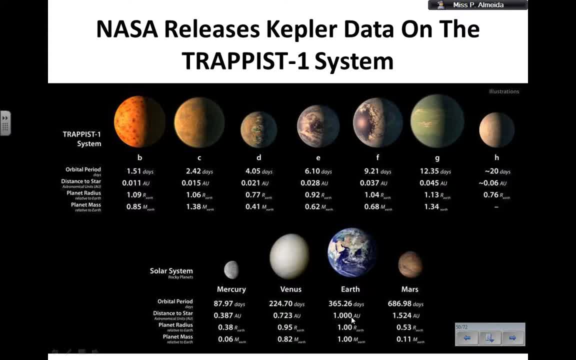 different than the planets that we are finding so far. they seem to be different from the earth. now, this system that then has the actual name of trappist system, trappist-1 system, has planets there are a little bit smaller, so closer to the type of size and composition that the earth has. but if 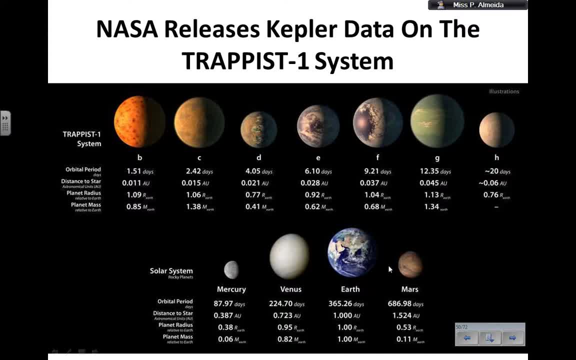 you compare. just you know, these are some of the planets in our solar system and these are the planets that are in the trappist system. and look, so let's speak. yeah, this one, for example, the orbit of the earth is different from the earth. yeah, this one, for example, the orbit of the earth is different from the earth. 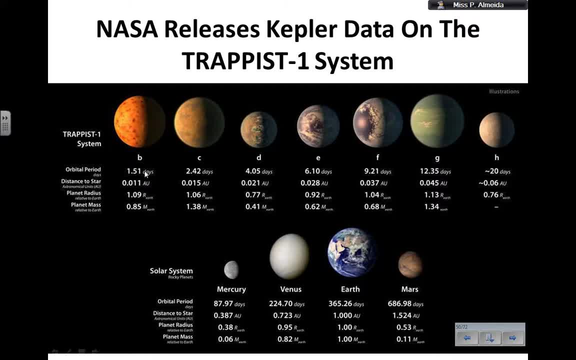 period 1.51 days: that's how long it takes to go around the star once okay. period 1.51 days: that's how long it takes to go around the star once okay. Barkery, the closest one to our star, is 87 points 97 days as an orbital period. 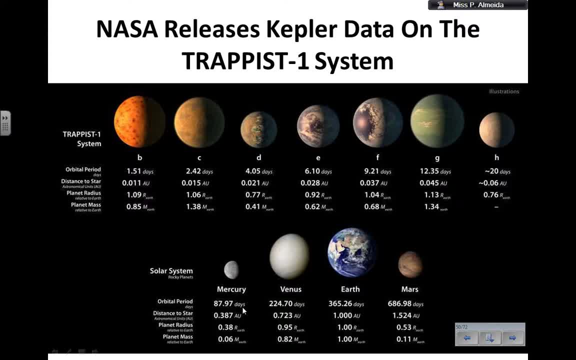 the closest one to our star is 87 points, 97 days as an orbital period. okay, so here are the distance to the stars. okay, so here are the distance to the stars. one astronomical unit is the mean distance between the earth and a planet, the Sun. sorry so if the earth is one, Mercury is not. point three: look at this. 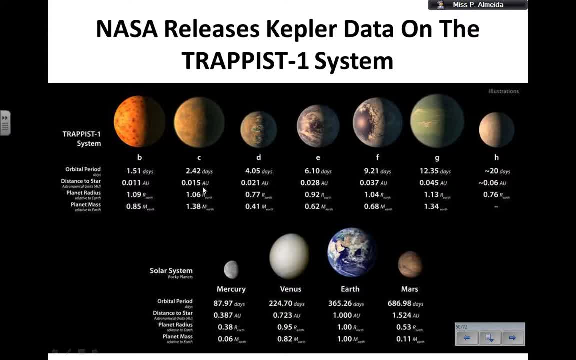 guys: 0.011, 0.015, up to 0.06, okay, so these are the type of planets that were found. okay, and this was a massive discovery because, as you're going to see in my next videos, 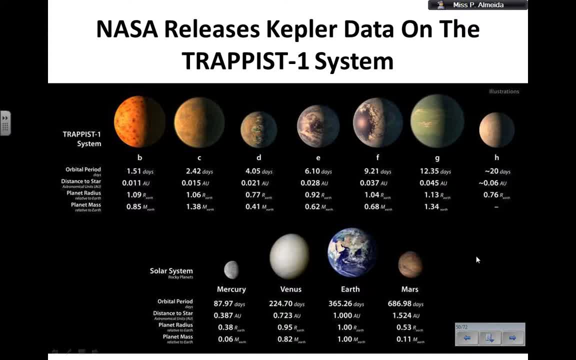 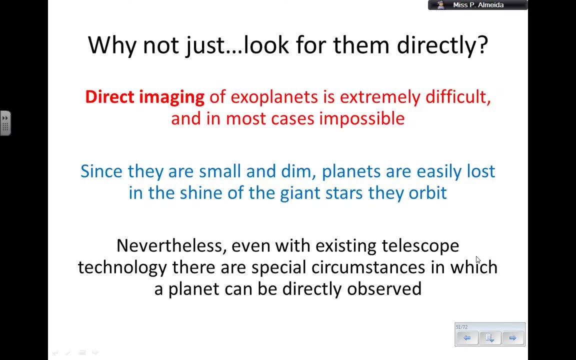 our techniques can be biased towards finding one or another type of planets, or planets that happen to be very close to the star, or planets that are very massive, and we're going to talk all about it, but this is just for your information, okay. so let's find about how do we find them? okay? 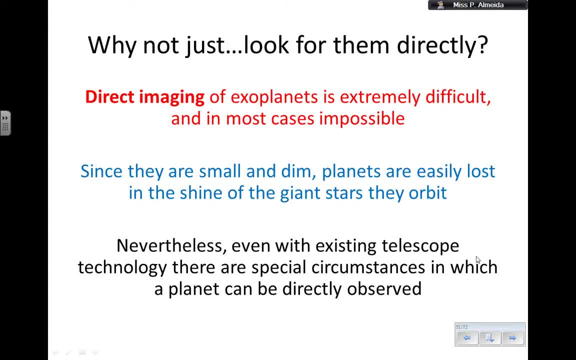 so let's find about how we get to know that these planets exist. so okay, there are planets around other stars. why don't we just look for them directly? you know why not now? the thing is, direct imaging of the exoplanets or extrasolar planets is very, very difficult, almost impossible. 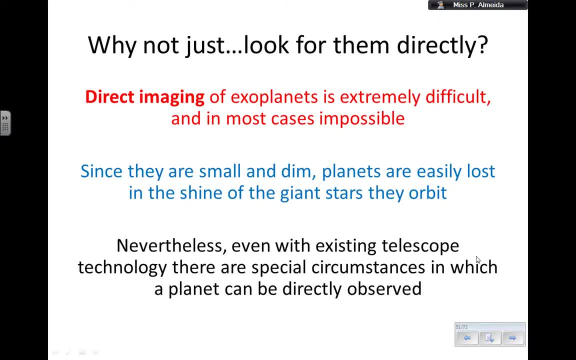 really because the planets are much smaller than the star. they are dim. they don't reflect a lot of light if they are very far away, or they may reflect a lot of light, but if they are very far away we don't see it. the planets are easily lost in the shine of the. 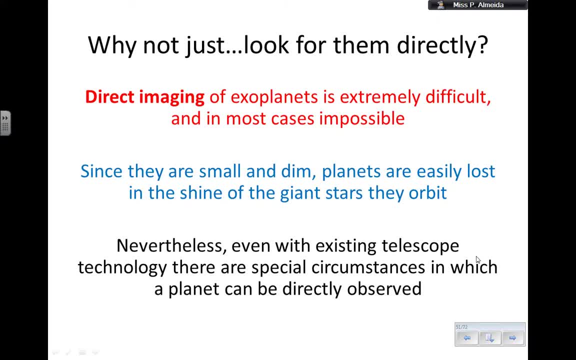 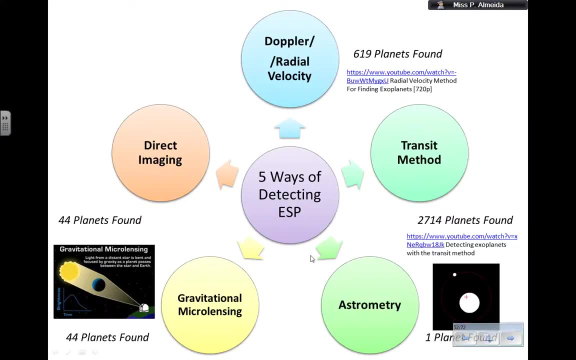 giant stars they orbit, so it's quite difficult, okay. however, even with existing telescopes, the technology, and there are special circumstances where I can actually find a planet directly. so these are some techniques that I'm going to go through with you, and today I'm going to focus on 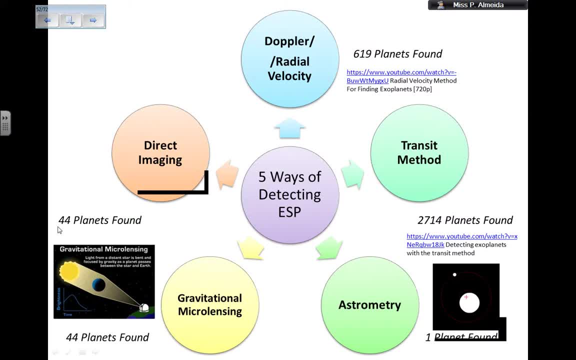 direct imaging where, up to when I did this PowerPoint, 44 planets have been found. I'm pretty sure this is now not up to date anymore. okay, so today I'm going to talk about direct imaging. there are other techniques, as you can see here: Doppler or radial velocity transit. 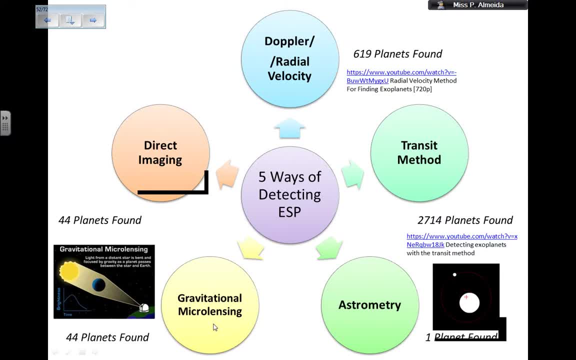 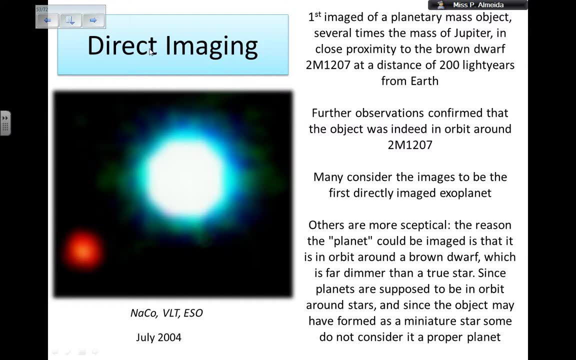 astrometry and gravitational microlensing. today I'm focusing on this one. okay, so direct imaging. the first image of a planet around a star we got it was in 2004,, so this had several times the mass of Jupiter. 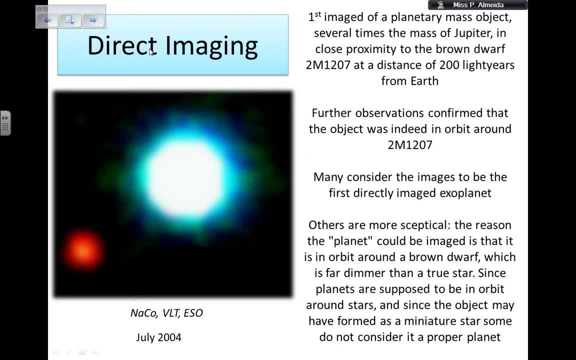 and it was very, very close of the white brown dwarf that it was around. so it was not a very shining star, if I can say that, also not very big, and the mass of the planet was huge, very close to the star and quite more massive than Jupiter, much more massive than Jupiter. 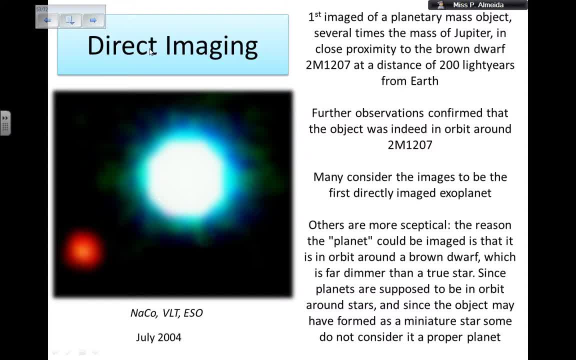 so this planet is about 200 light years away from Earth, okay, and then one of the things that you need to do is: okay, you believe there is a planet there, but you actually kind of need to confirm. so further observations confirm that it was indeed a planet. okay, so this is what is considered to. 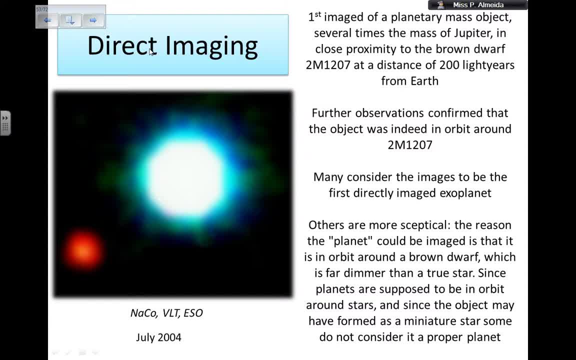 be the first image of a directly imaged exoplanet. okay, now other people say it could be just that. you know, the reason the planet could be is that it is. it is around orbit, around dwarf, which is far. 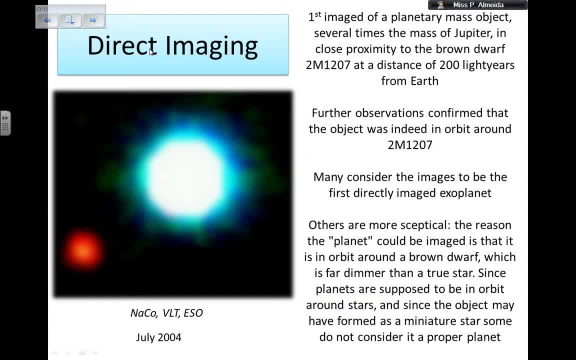 dim under the true star. so planets are supposed to be in orbit around stars and since the object may have formed as a miniature star, some do not consider it to be a proper planet. they say: how do you actually know? but this is, you know. we're focusing on the actual, direct imaging. 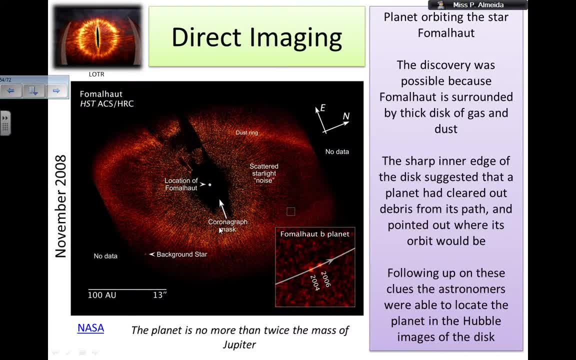 and this is more or less how it looks like, and please see the similarity between this and the eye in the Lord of the Rings. okay, so what happens is the following: I have a star right here at the center, okay, and what is? 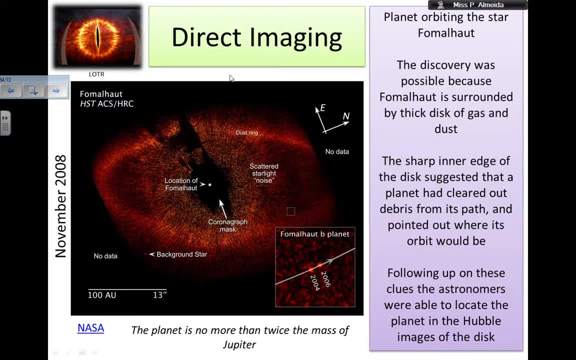 going to happen is the star, especially when it's a young star. it has a lot of dust and particles around it, okay, and planets? the way that they form is that they accrete, they gather up that dust and those particles through gravity and then, because of conservation of angular momentum, 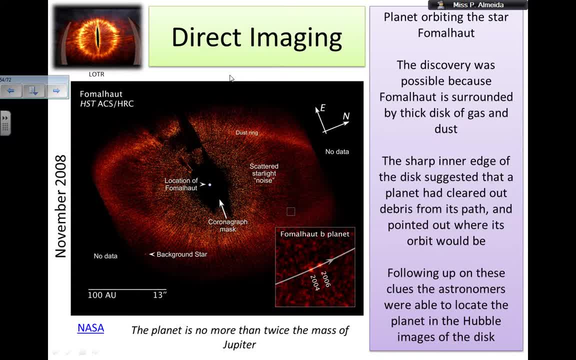 they become spherical and all that stuff. so what happens is if I have a planet I'm going to have and if I'm trying to look about this planet directly, I can look at the disk and then, if I have- which you may not see well in the image, but if I have this part in here- 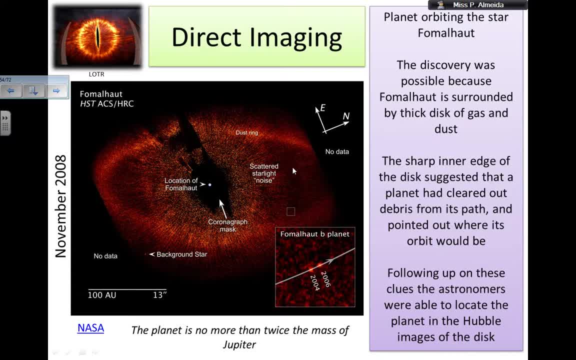 where the disk is a little bit more clear. it looks like there is an object in there that is clearing up space, is clearing up dust and particles. so you're like, hmm, there could be a planet in there. so what they do is they keep looking at that planet or that place. 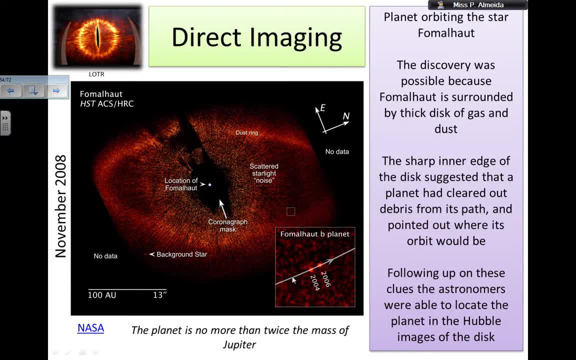 that orbital body. and then this is the zoom in images. in two years you can see that this body is actually moving around the star. okay, so this discovery was possible because this star has thick disks of gas and dust, okay, and then the sharp inner edge of the disk suggests that the planet 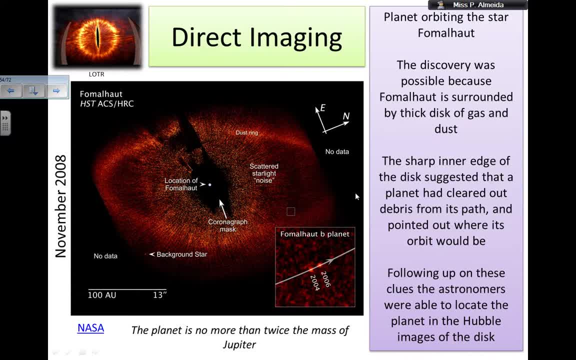 had been clearing out the derbies and then- maybe I don't know, maybe it's because of the- we could have a place where the orbit would be okay. and then we need to follow up on our clues. we need to look, using other techniques maybe, or trying to look at this state and trying to find. 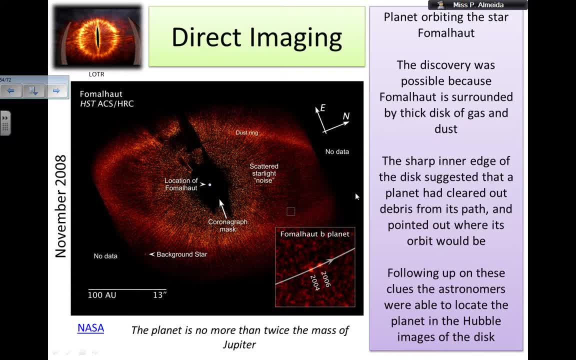 out if it could really be a planet. so we can use other techniques to confirm or to get more information, or we can keep using the same one if we cannot have any other way to find out that there is a planet with another technique. but keep an eye on them. okay, it takes a long time. 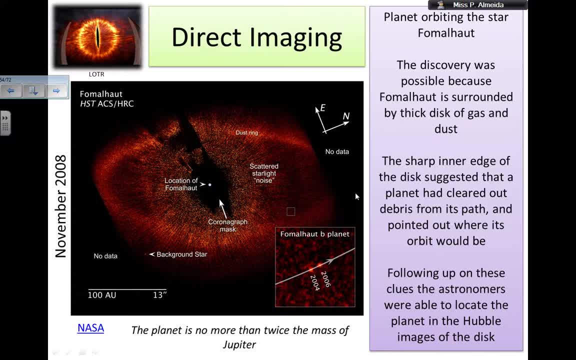 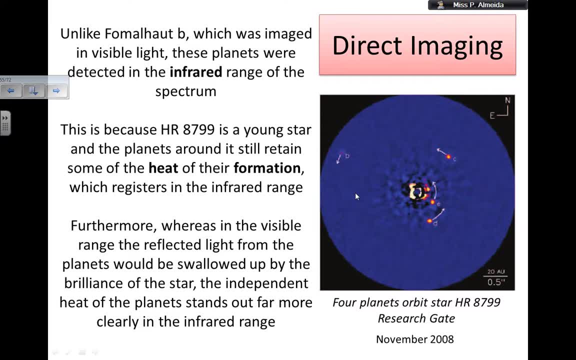 until we actually say: yes is a planet, but this one is okay. so direct imaging, okay. now, most times you find a planet through infrared. okay, that one, the one that i showed you before, was found using visible light, but actually normally you use infrared. and this is because, when you have 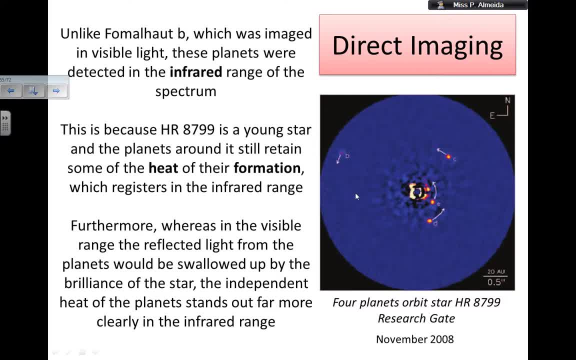 a young star and you have planets around this star. they still have some heat from their formation. okay, and as you know, okay, and as you know, okay, and as you know already, infrared is, um, the best wavelength really for me to pick up the heat. okay, the amount of 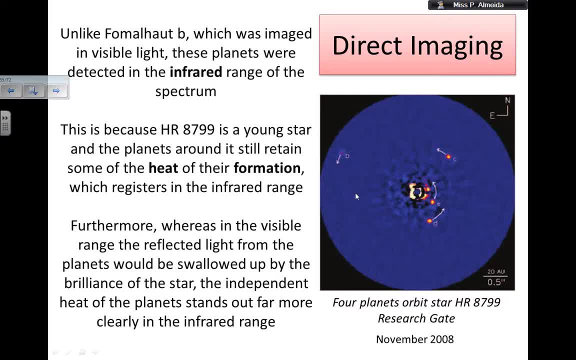 thermal energy. something has all right. so the visible range is, uh, the reflected light from the planets would be shot as well. um, swallowed up, really- i was trying to say another word- but by the brilliance of the star, and if you have the heat of the planets, this is going to stand out. 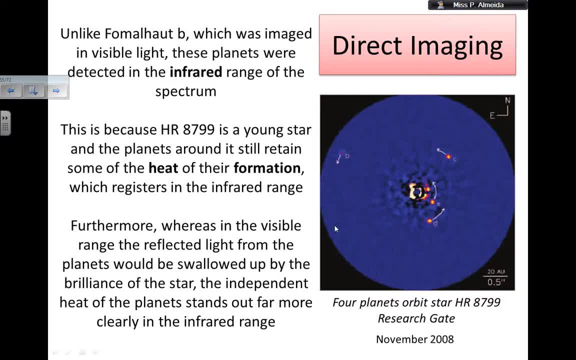 more, uh, in the infrared range, and this is another example. so this is a four or planets orbiting this star. okay, and this is from november 2008. i have the star in here, but also i have this thing in there, this thing in there, this thing in there and that thing in there. 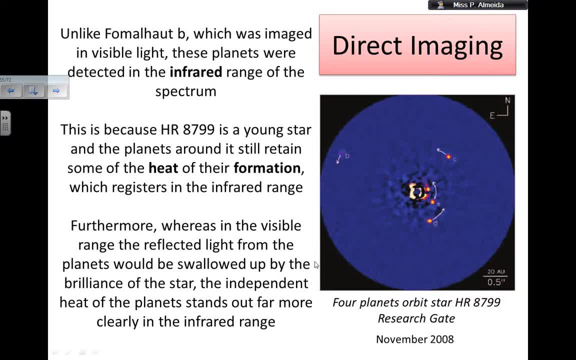 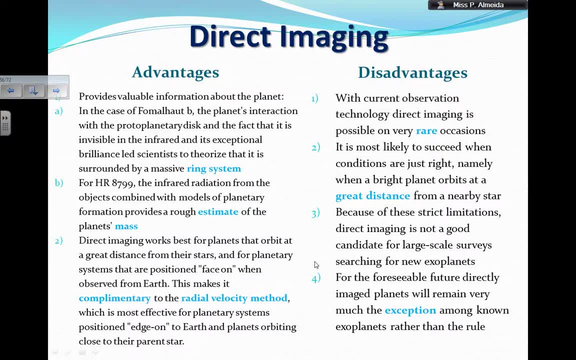 okay, and they happen to be planets, so direct imaging does work, uh. however, you need to have certain conditions, okay, so let's just wrap up this with advantages and disadvantages. so, for example, it provides valuable information about the planet. i mean, it provides valuable information about the planet. i mean. 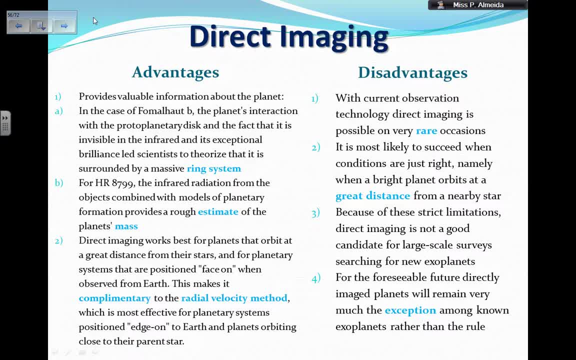 what is the best way to get to know about something if you if not looking at it directly? right and then, oh my god, and then, uh, in the case of the star, that star that i showed you in the second slide, uh, not the second slide- the second type of planet, the one with the lord of the ring. 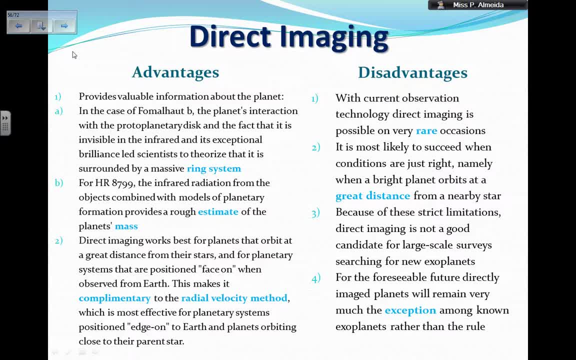 eye. the planet's interaction with the disc and the fact that is invisible in the infrared um led scientists to make a theory that maybe is surrounded by massive disc uh ring system. so again, you can look, if you look at where other wavelengths and if you're lucky. 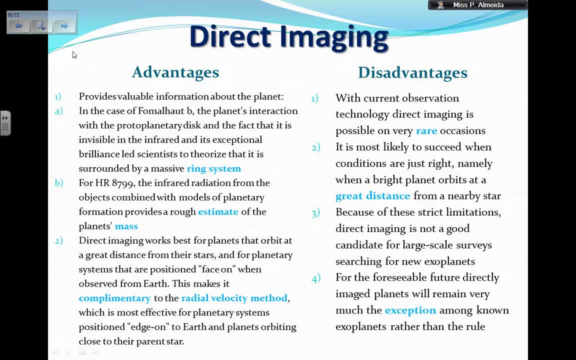 enough to be able to see the planet in other wavelengths. you can gather out or make theories about more information about that planet. okay, does it have a ring system? so the other thing is: uh, if you combine the infrared radiation with models of planetary formation, so using like 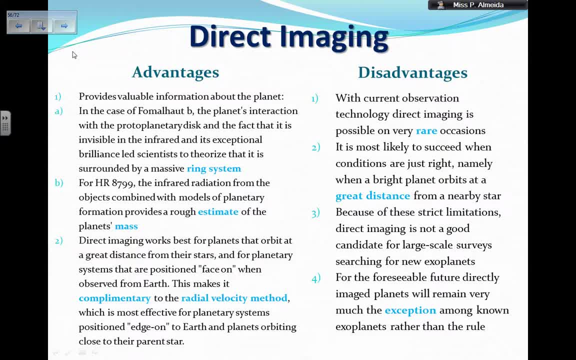 really advanced mods, you can get a rough estimate of the planet's mass. and that's amazing because- Because there is kind of a focus for people to try to find smaller planets- Most of the planets we have been finding before were very, very massive. I mean about twice to five times, ten times the mass of Jupiter. 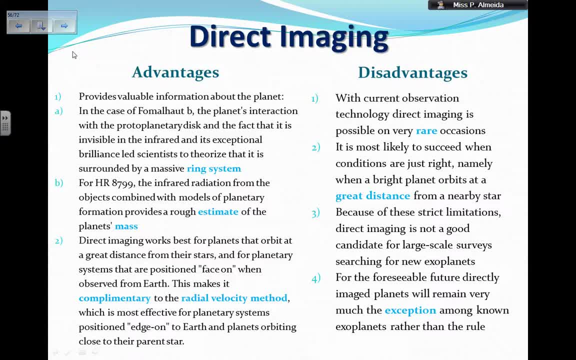 And people are kind of looking for other planets like ours, So that's amazing, okay. Also, it works best for planets that orbit at a great distance from the stars. okay, And I also need the planetary system to be positioned face-on when observed by the Earth. okay.